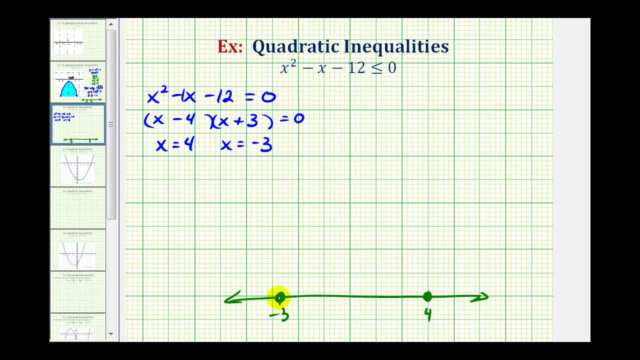 Notice how we've now formed three intervals on the number line. We have the interval on the left, the interval on the middle and the interval on the right. And for perspective, let's go ahead and put a zero here. Now we're going to find a test value in each interval. 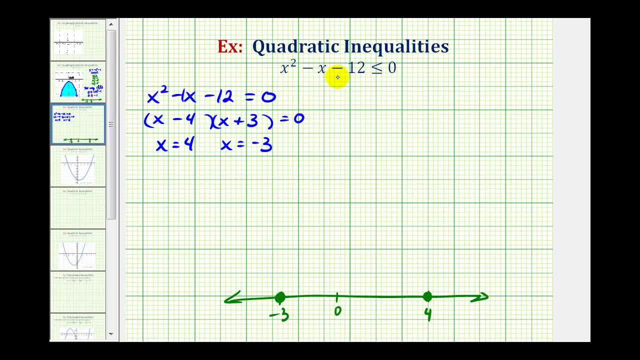 and test to see if it satisfies the original inequality. If the test value satisfies the inequality, then the entire interval is part of the solution. If the test value does not satisfy the inequality, the entire interval is not part of the solution. So for our test values, 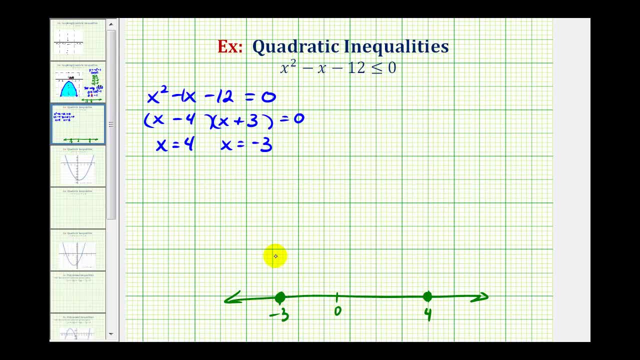 we can't use the points that we just plotted. So to the left of negative three, let's use negative four. In the middle, let's go ahead and use zero, And to the right, let's use five. So let's go ahead and test these in our inequality. 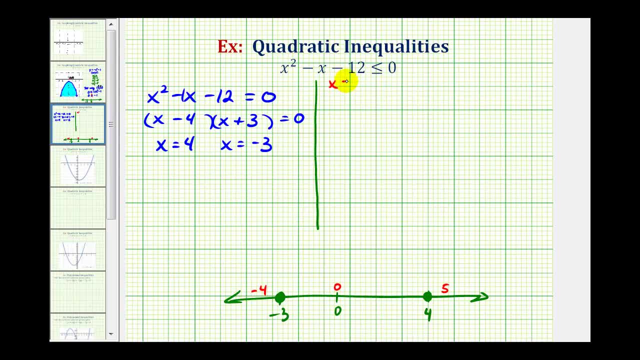 We'll first test: x equals negative four. Well, when x is negative four, we would have negative four squared minus negative four, minus 12 less than or equal to zero. So right now this is a question. we're not sure This will be positive 16 plus four. 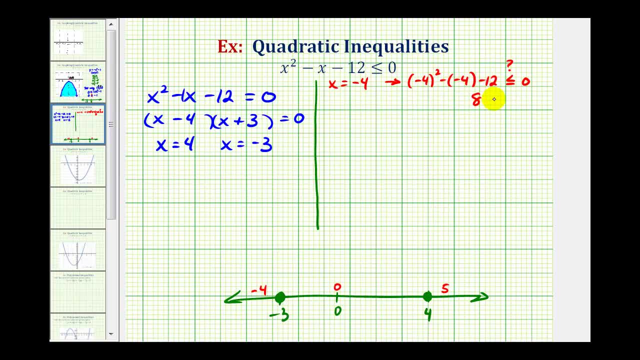 that'll be 20 minus 12,, that's eight. So we have eight less than or equal to zero. Well, eight is not less than or equal to zero, so this is false. So the entire interval to the left of negative three is false. 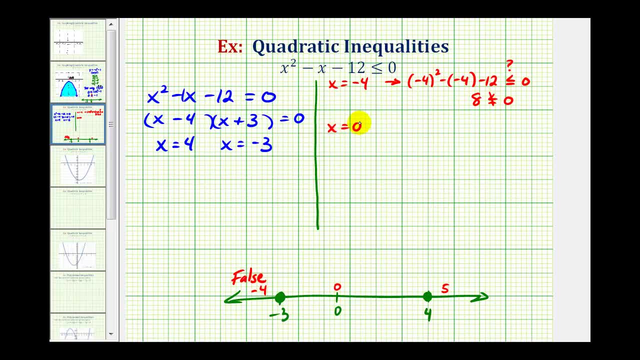 And now we go to the next test value. Let's test x equals zero. Well, if x is zero, we're just going to have zero minus zero minus 12, or negative 12 less than or equal to zero. This is true, which means the entire interval. 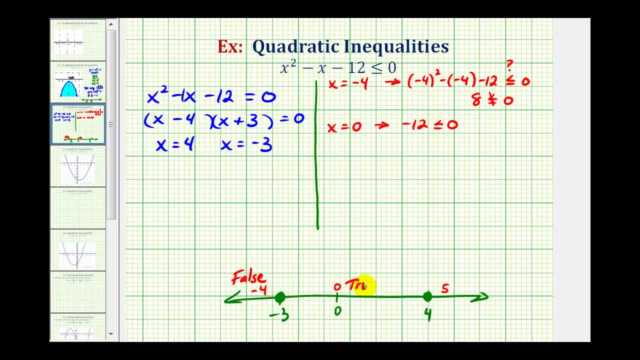 from negative three to positive four is true. So let's go ahead and graph this interval from negative three to positive four, including the end points. Now we'll test. x equals five, So we would have five squared minus five, minus 12, less than or equal to zero. 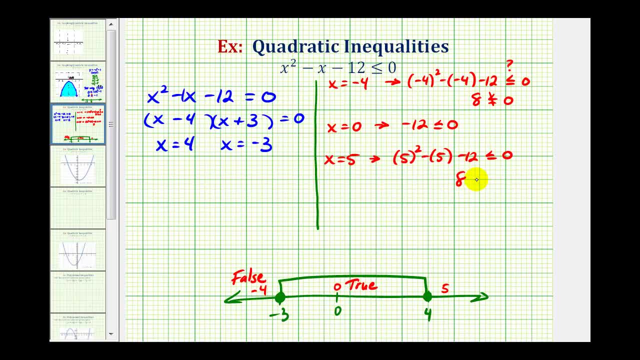 25 minus five is 20,. 20 minus 12 is eight. Eight is not less than or equal to zero. So the interval to the right of four is false. So we're going to test: x equals zero. So the closed interval from negative three to positive four. 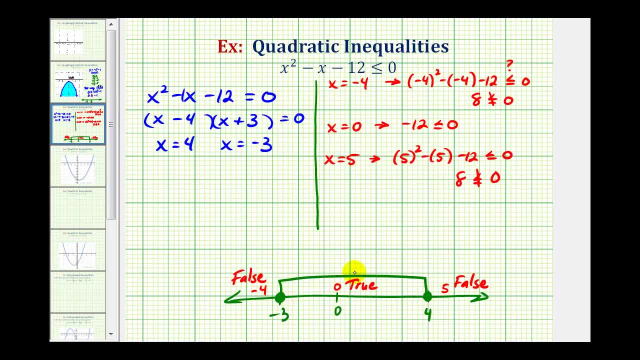 is the solution to this inequality, which means any value in this interval would satisfy this inequality. Let's go ahead and state this solution a couple other ways. Again, here's the graph of our solution. Using interval notation, we'd have the closed interval. 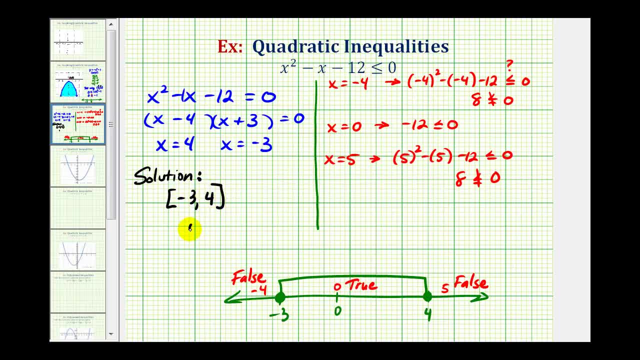 from negative three to positive four. or we could also say: x is greater than or equal to negative three and less than or equal to positive four. And, as I mentioned at the beginning of the video, we can actually solve this quadratic inequality very quickly by graphing the function f of x. 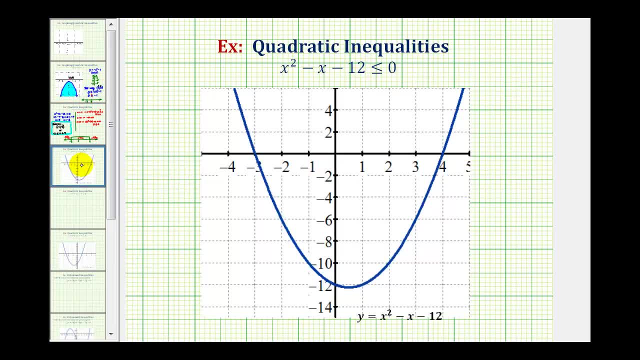 equals x squared minus x minus 12.. So here's a graph of f of x equals x squared minus x minus 12, or, if you want, just y equals x squared minus x minus 12.. Since we want to know when x squared minus x minus 12. 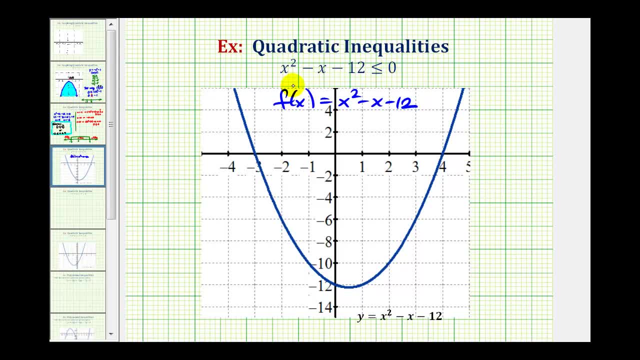 is less than or equal to zero, we can use this equation. So we're going to use this equation here. This is less than or equal to zero. That's going to occur when the function is less than or equal to zero. Remember, function values. refer to y values. 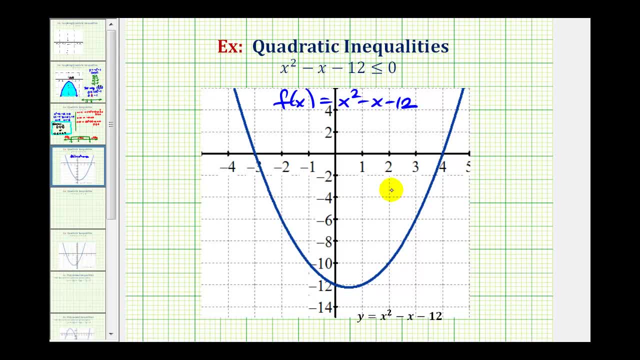 so, when the y values are less than or equal to zero, the function is on or below the x-axis, which would be this piece of the graph here, And notice: this occurs along the x-axis from negative three to positive four, and this interval is the solution. 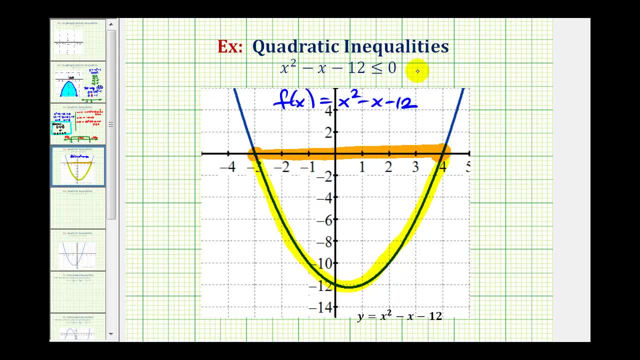 to our quadratic inequality. So while the process for solving these by hand is pretty involved, solving them graphically is very straightforward. We'll take a look at another example in the next video. 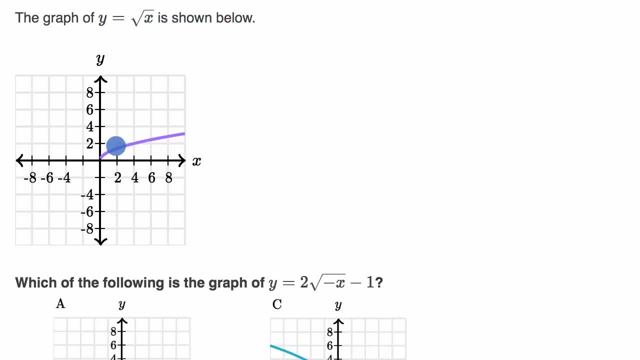 We're told. the graph of y is equal to square root of x is shown below. fair enough, Which of the following is: the graph of y is equal to two times the square root of negative x minus one. And they give us some choices here. 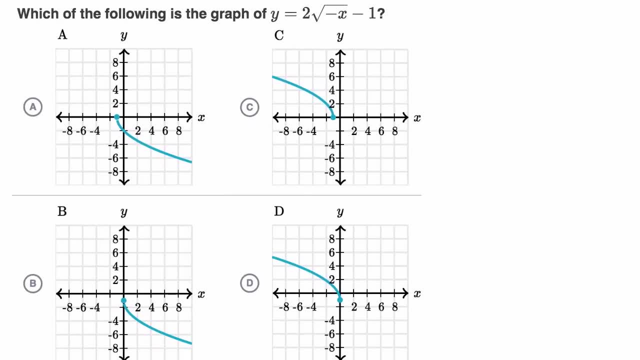 And so I encourage you to pause this video and try to figure it out on your own before we work through this together. All right, now let's work through this together, And the way that I'm going to do it is I'm actually going to try to draw.